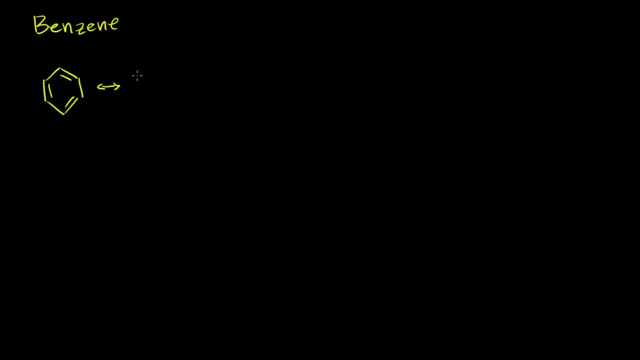 And it's not its only configuration. Sometimes it's shown to be in resonance with this form right here, So the double bonds all flip around the circle like that. Or sometimes it's simply drawn like this- And I talked about this in the last video, just to show that. 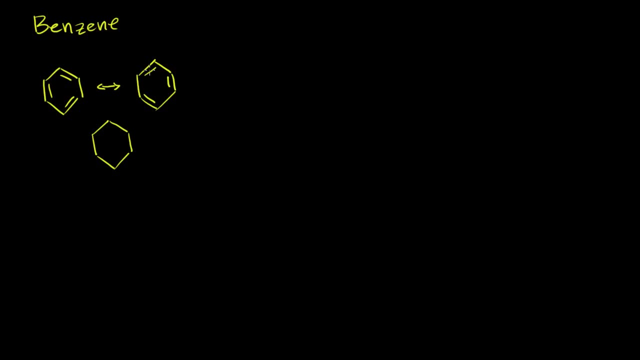 really neither of these configurations is exactly right- that these pi electrons are just moving around the entire circle, The entire ring. So sometimes you'll just have the hexagon with a circle on the inside to show that the pi electrons are just floating around the entire ring. 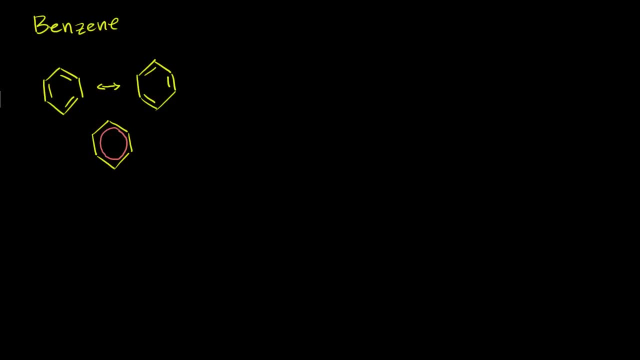 Now, if I were to add something to the benzene ring, it's pretty straightforward to name it. So say, I have this molecule right here, That's benzene, But let's say this carbon over here. it has one, two, three. 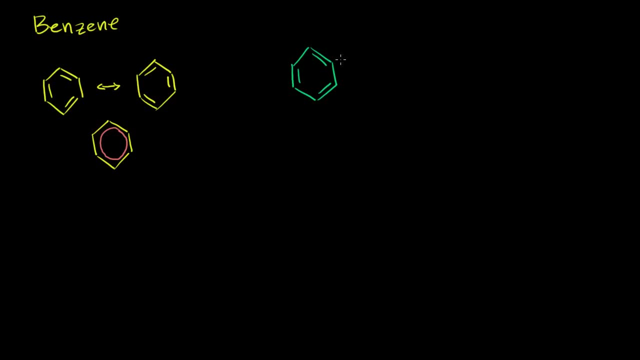 bonds. If I didn't draw anything else, you just assumed that there's also a hydrogen here. But maybe there's something. Maybe there's no hydrogen there, Maybe- let me do this in a different color- maybe you have a chlorine there. 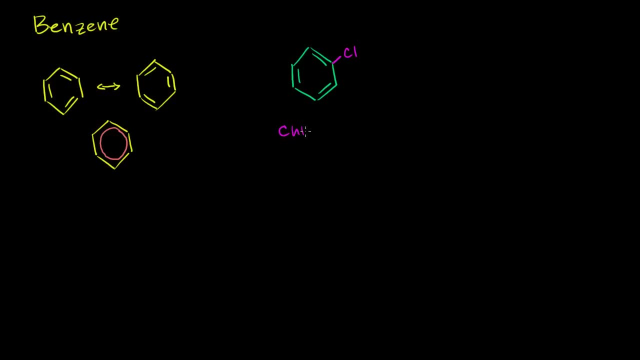 Well, this is just chlorobenzene. If that was a bromine, it would be bromobenzene. So pretty straightforward. If let me draw it, let me change it a little bit. Let's say you had a chloro there, and let's say you had a. 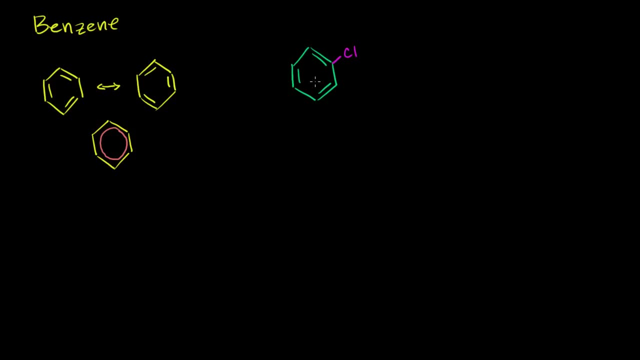 bromobenzene? Oh, I don't know. Let's say you had a bromo over here. Let's say you have a bromo over there, Draw the bromo, So you could just start numbering. You could actually start numbering in either place. 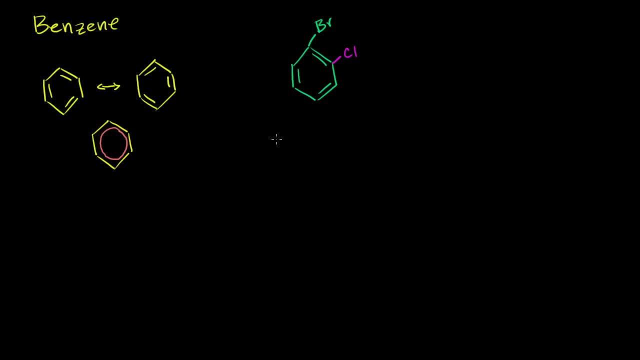 Let's start with the bromine. It's alphabetically in front, So this would be one bromo, two chlorobenzene- Pretty, pretty straightforward. Now it gets a little bit more involved. The IUPAC, which we know, is kind of the group that named 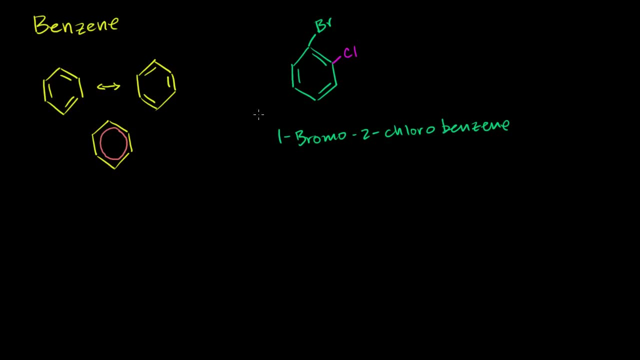 most things. they tend to everything else we've seen so far. they came up with a separate naming mechanism from the common names. But benzene- it's so ingrained in the organic chemistry community that all of the benzene or benzene derivative 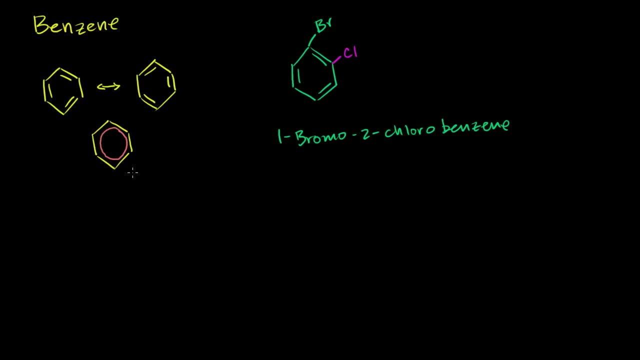 molecules. they just kind of said: well, you know what, we're just going to use the names that everyone uses. So here's a couple of common benzoic molecules, Common benzene derivatives. So if you have this molecule right here, let me. if you. 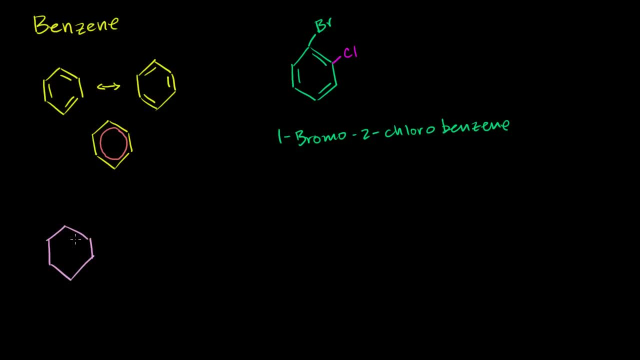 have this molecule right here, I'll actually draw the pi electrons as a circle. Actually I'll draw it with the double bonds. So let's say: you have this molecule right here and over here you have an OH. You have an OH right there. 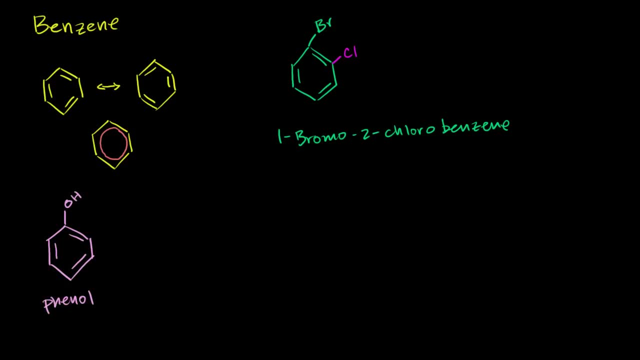 This is called a phenol. This is called a phenol, So it's not called benzene anymore. And if you had a molecule that looked like this, if you had a molecule that looked like this, so just like a phenol. so essentially it is a phenol, but 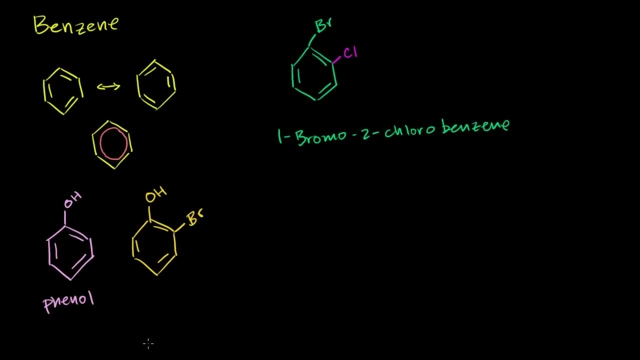 let's say you have a bromine right there. What you do is you start numbering at the group. that's making this a phenol. So you start numbering there 1, and then you get to the 2. So this is 2-bromo-phenol. 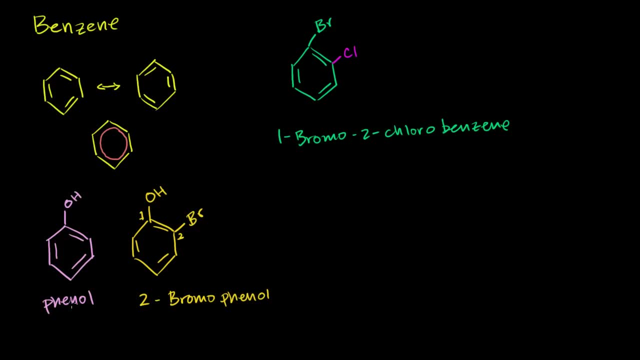 And unfortunately this is one of those things that you just kind of have to memorize- that a phenol is really just a benzene ring with an OH group, Another one that is probably a good idea to memorize, at least for me, in organic chemistry the most confusing thing is 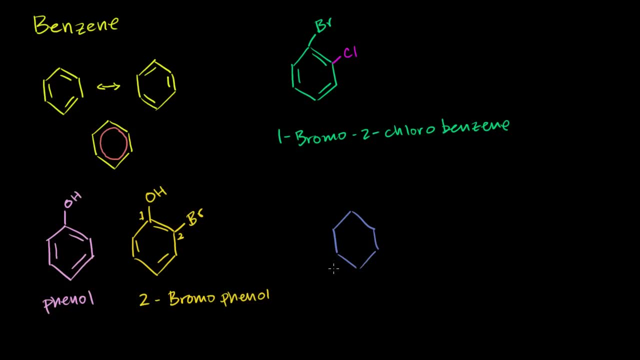 when someone says the name of a molecule that it sounds like they expect you to understand, but you don't understand it. So it's, I guess, a good idea to understand as many names as possible. So if you just have a benzene ring and you just have a, 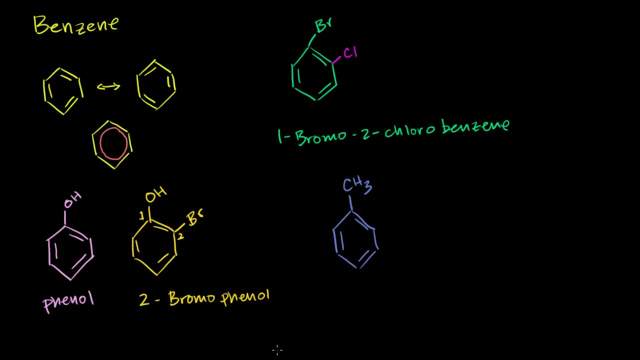 methyl group. You just have a phenol. You just have a methyl group attached to that benzene ring. This is called toluene And once again, if you had a- let's say you had a fluorine right over there- this would be 1,, 2, 3-fluoro-tol-luene. 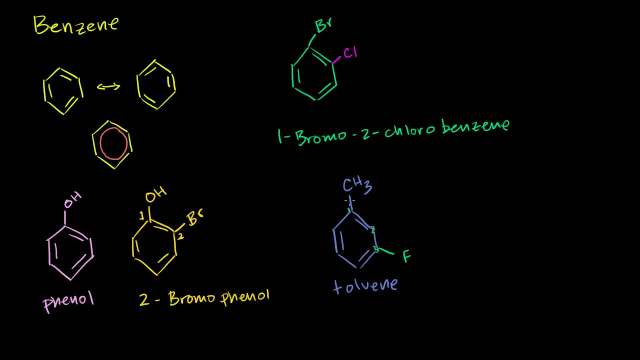 I always have trouble saying that, Because 1,, 2, 3. You started the group. that's kind of making this the toluene, And so let me make it a little bit clearer. So this would be 3-fluoro-tol-luene. 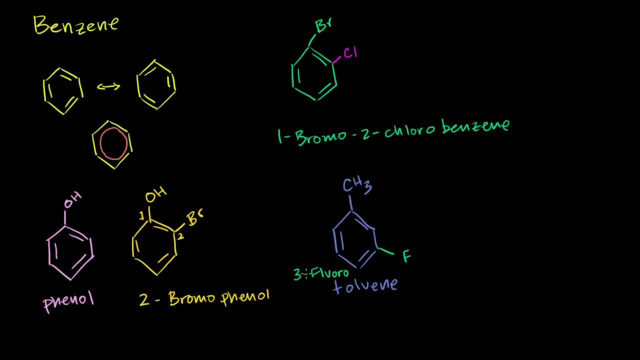 This would all be in one word. I just wrote it up here to save some space. Now a couple of other ones that you'll see And once again, as you know, if you watched many, many Khan Academy videos, I hate memorizing things. 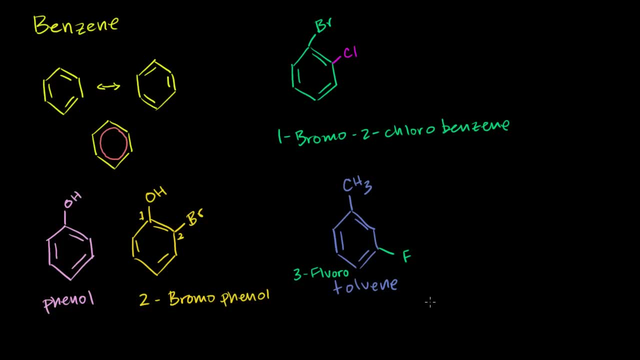 But these are just names And these aren't systematically derived. The chemistry community just uses them because that's the way they've heard them. So it is one of those things you kind of have to memorize. So if you have a benzene ring where the functional group 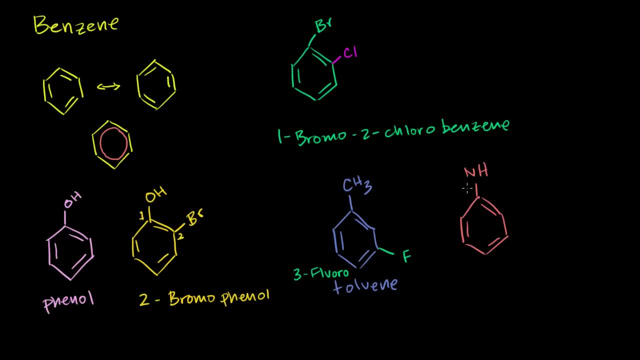 that's kind of defining the benzene ring. it's essentially becoming an amine. We haven't actually covered videos on amines yet And I'll do that in a future video- But essentially it's replaced one of the hydrogens in ammonia. 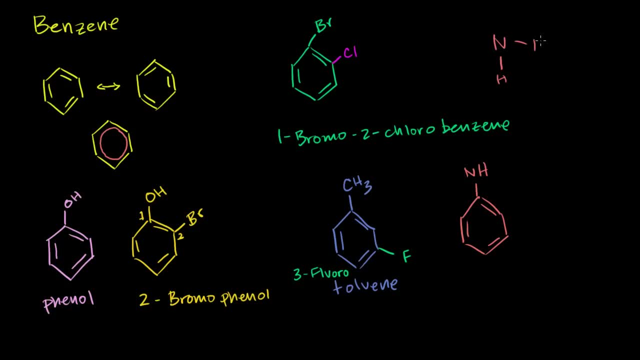 Ammonia has three hydrogens and one lone pair. Here we've replaced one of the hydrogens. Actually there's two hydrogens. here We've replaced one of the hydrogens with a benzene ring- This type of thing. you call it aniline. 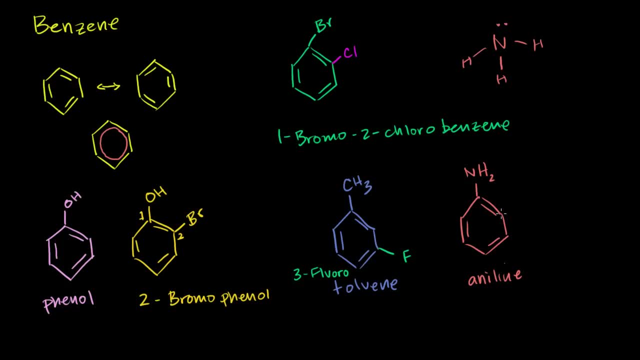 Right there, And the same idea. If I put a fluoro here, this would be 2-fluoroaniline. So you use whatever the base molecule is and then you just name it really the way. we've named a lot of things before. 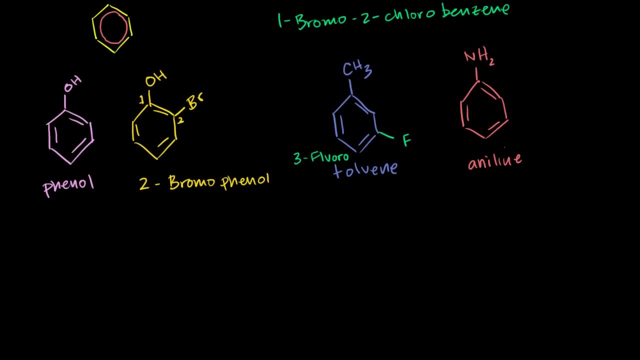 And I'll just introduce you to two more, just so that you have them under your belt, so that you will have seen them before if anyone introduces them to you- And they're really introducing groups that we'll study in more detail in the future. 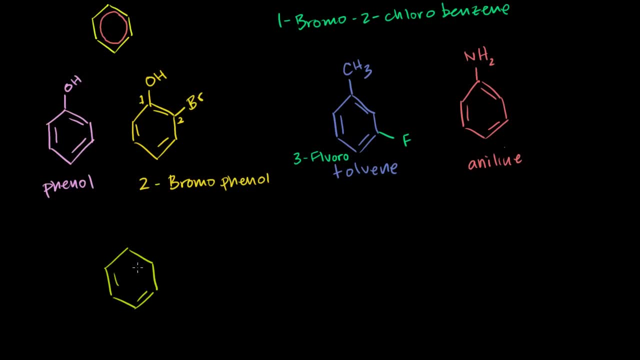 But if you have a benzene ring once again, So we have a benzene ring And then you have a carboxyl group, And we'll talk more about carboxyl groups in the future. But it creates carboxylic acid. 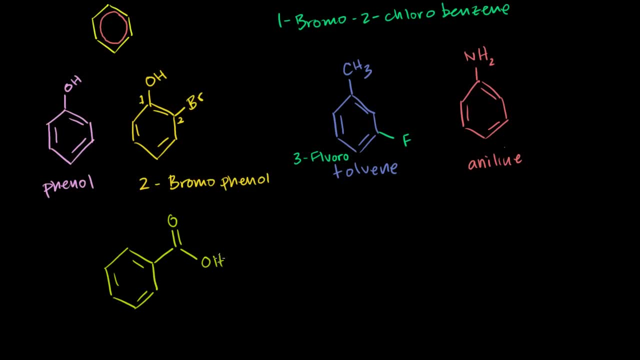 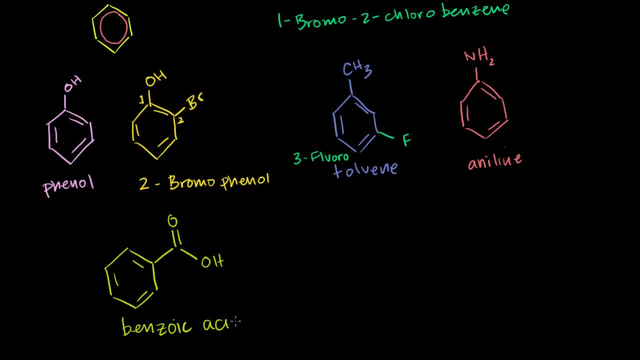 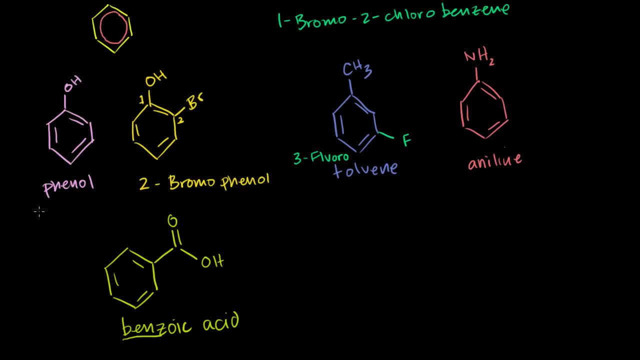 You have the benz part for the benzene, So let me make this in different colors: The benzene part that gives us the benz right there, And then in general, whenever you have a carboxyl group like this, it becomes a carboxylic acid.